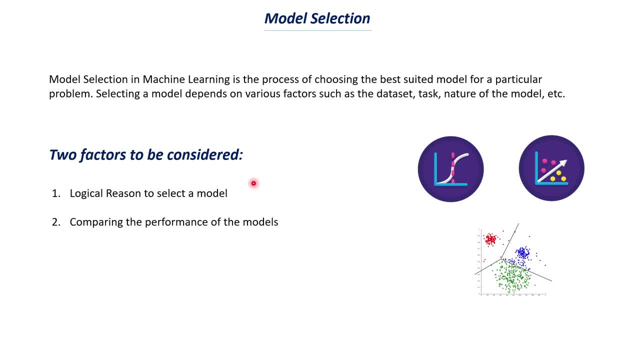 performing this model selection. The first thing is: what is the logical reason, you know, in order to select a model, So why we have to choose a particular model in a particular case. So we will discuss about this first one in today's video, And the second one is about comparing the performance of the models. So this is what we will try to do in Python in the next video. 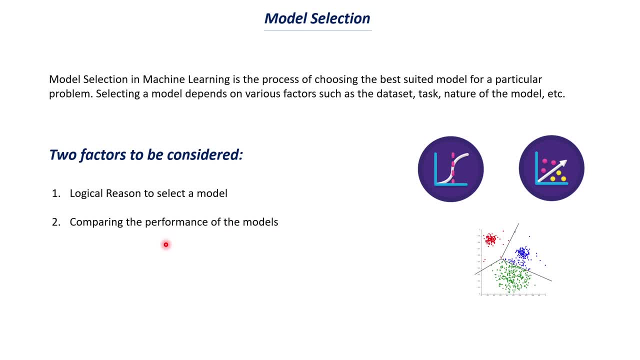 Okay, so it is just comparing how the different models are performing for that same data set. So we can do this comparison in Python. So we will focus on the first part in this video And then we move on to the yo, the second part in the next video. Okay, so so when we talk about this model selections, models can be selected based on two important factors. 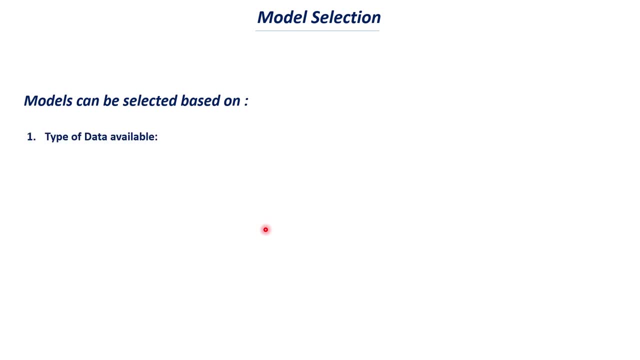 One is the type of data available And the next one is the type of the task that we need to carry out. Okay, so if we talk about the first one, which is selecting the model based on the data that we have, So usually when we have image data and video data, we use CNN. 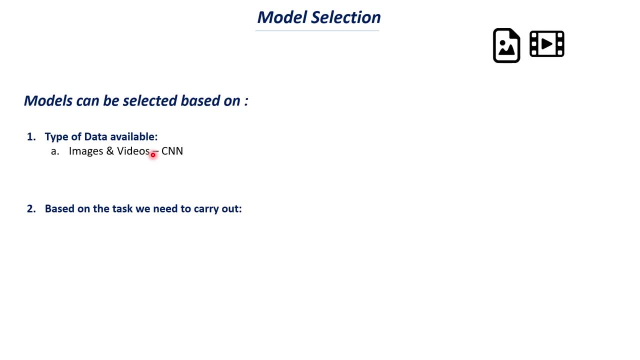 So CNN stands for convolutional neural networks, and convolutional neural networks are known events that we sort of track. Thank you for listening to this video. If you like my opinion, please subscribe to my channel and also click on the bell button. See you in the coming video. 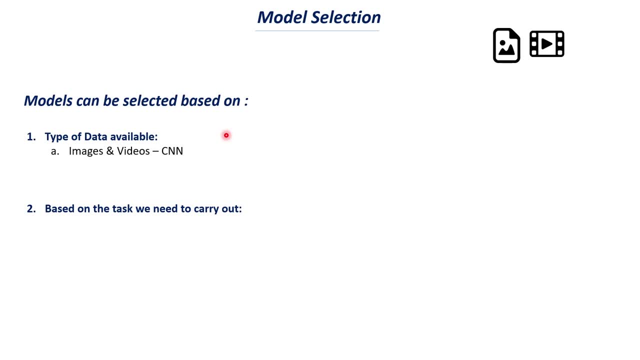 for image recognition and this computer vision tasks, and again, so video is nothing, but they are like several images, that that are present in frames. so like videos are nothing, but they are basically images. so for image data and video data, so we, like cnn, are the best suited models and when 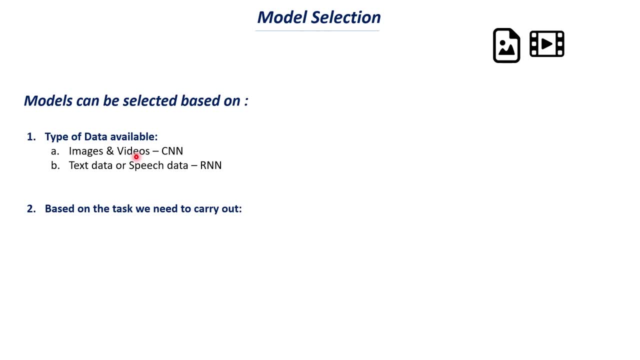 you add this text data or speech data. in that case we use rnn, where rnn stands for recurrent neural network. so all these things comes and comes in the deep learning part, and we will discuss about the cnn and rnn in the deep learning course and and we will also be working on 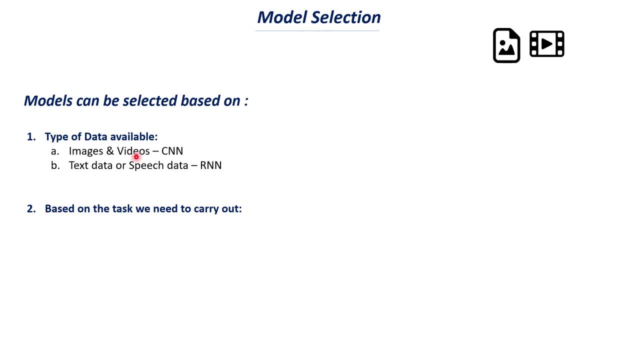 several deep learning projects along with this machine learning course. so in that you know, you will understand. so how the cnn works, so we can use them, and how this rnn works and so on. and generally, like when it is numerical data, we go with the machine learning models, like logistic. 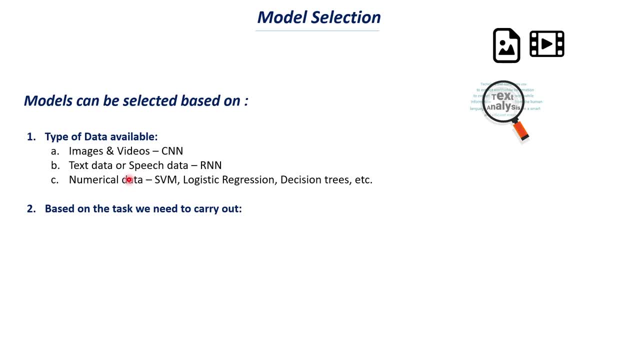 regression support and machine decision trees and so on. so it is not that we can apply only machine learning models with numerical data. we can also use neural networks as well for numerical data. but so generally we will go with machine learning model itself when the data is like simple, like neural, like numerical data, whereas if you consider image data and text data, 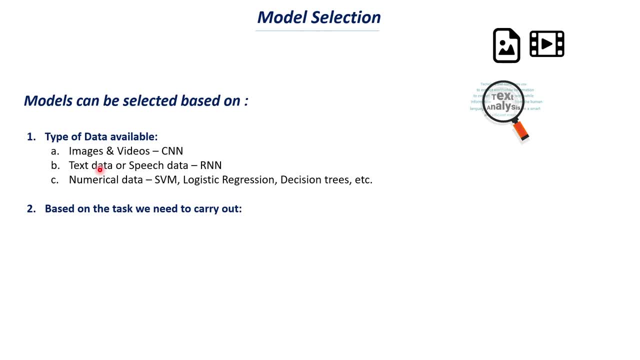 the data is kind of complex and it is. you know, there is like a huge amount of data has to be processed and has to be learned from. so that is why we move with deep learning for this image and text and speech type of data, with deep learning and and work on this spm, logistic regression and 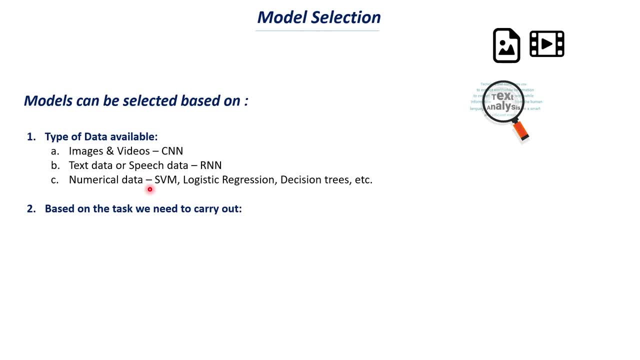 these kinds of simple machine learning models, when it is numerical data and the second you know like based on the task, how we can select the model. so if we talk about this, so classification task, we use the models like support vector, machine classifier, logistic, regression, decision trees, etc. 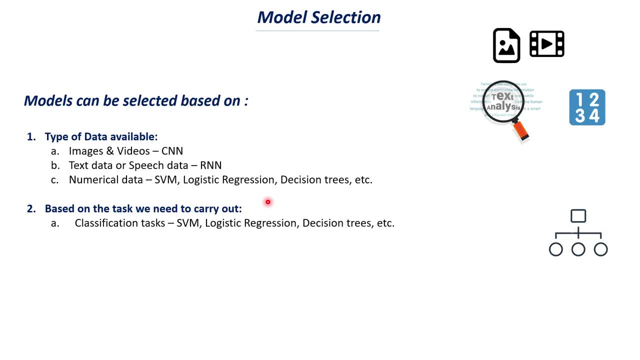 so we know that classification task. we will try to classify the data point into different classes or categories. okay, so logistic regression is a pure classification model, so you cannot use use it for regression. so it has this name called as logistic regression because it is developed from linear regression. so that's why this has the. you know it has the name logistic regression. 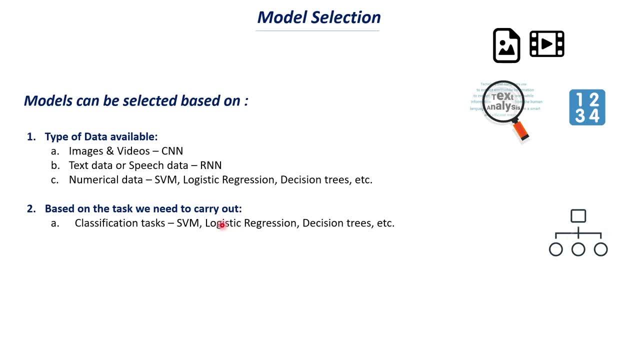 but actually it is used only for uh classification, whereas if you consider a support vector machine, so support vector machine it has both classifier as well as regressor again. so we also have models like random forest classifier, which can also be, you know, we also have a regressor based on random. 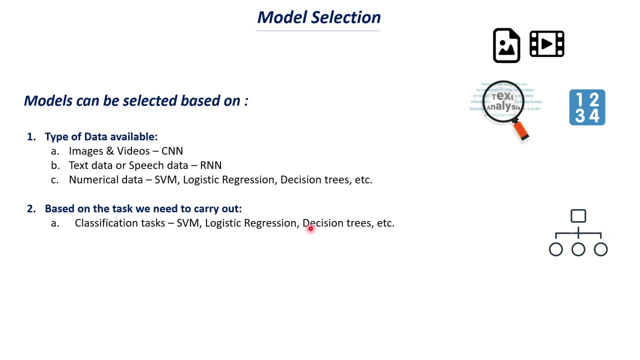 forest. so, like most of the models, can be used for classification as well as regression. but logistic regression is mainly used for classification and another important thing is logical regression is widely used for binary classification problem. binary classification in the sense when you have two classes or two categories. it's not like, uh, every time you will get best result, but if you 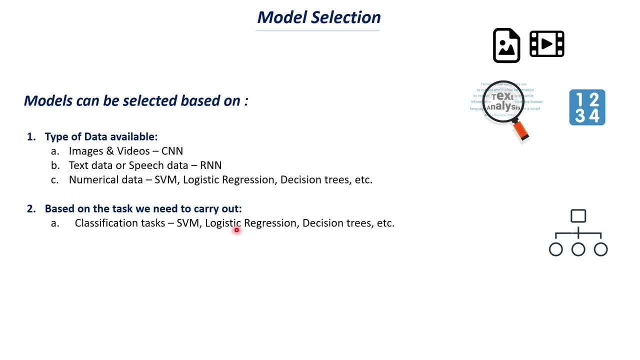 have a linear data and if you have a binary classification problem, in that case logistic regression kinds of works best. okay, and uh, if we consider support vector machine, it kinds of works well when the dimensionality of the data is like when you have, you know, uh, several number of. 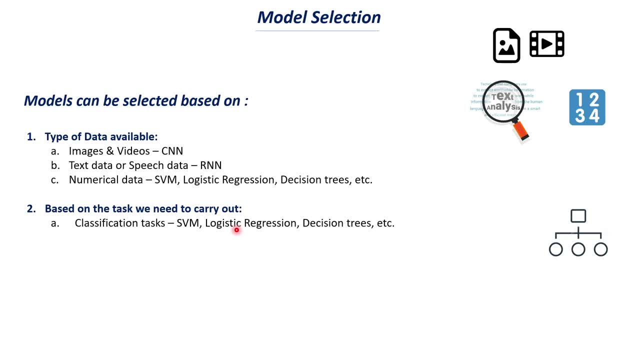 columns in your data set. so in that case support vector machine is the best suited uh model for your work and uh regression test. so if we talk about regression tasks, we have models like linear regression. so we also have random forest regressor and so on, so we also like support vector machine. 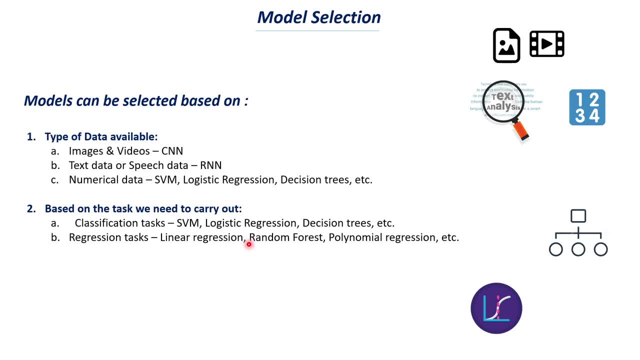 regressor, but you know, so, in general, random forest regressor it kinds of gives you better results because it is an ensemble model and it is, like you know, widely used. so we have linear regression, random forest regressor, polynomial uh regressor and so on. so, apart from this, you have kn and 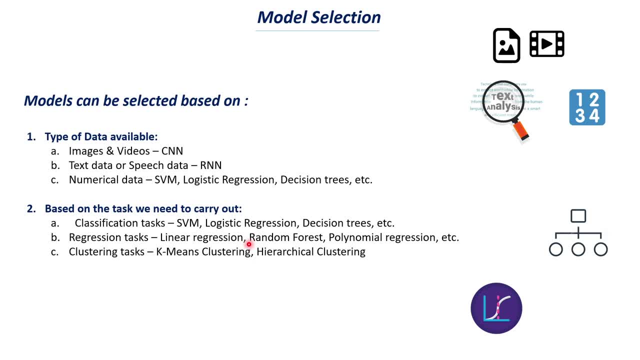 classifier came regressor as well. so these models are also there and if the task that you are performing is a clustering task, so obviously we have to go with. k means clustering and hierarchical. these are unsupervised uh learning models where we don't need labels at all. so these models will 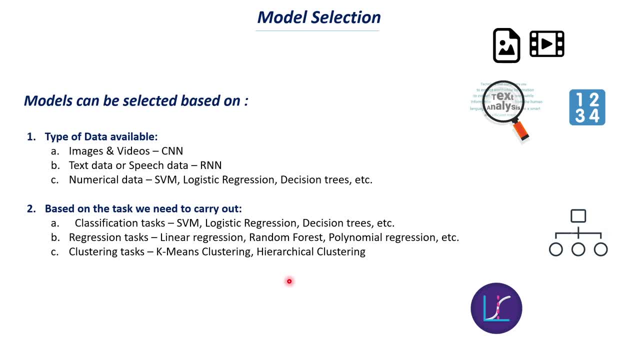 try to group the data based on their similarities and so on. so these are like two important things that you can consider. so if, uh, you know, so the thing is, you can choose your model based on the data that you have and based on what is the task that you want to follow. so these are like few. 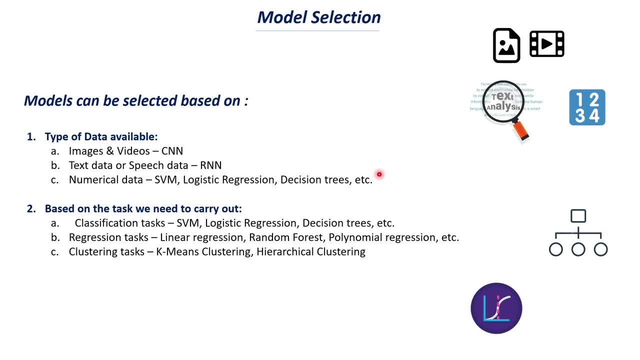 factors upon which you can select your model. so, apart from this, you have to understand about the advantages and disadvantages of all the models in machine learning. so once you understand this, it will give you a clear picture of which model to use when. so i'll just take three models and 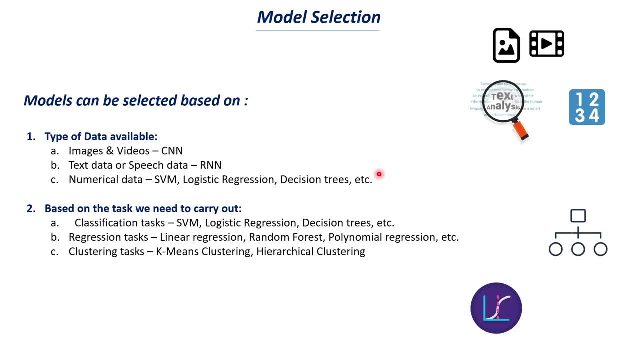 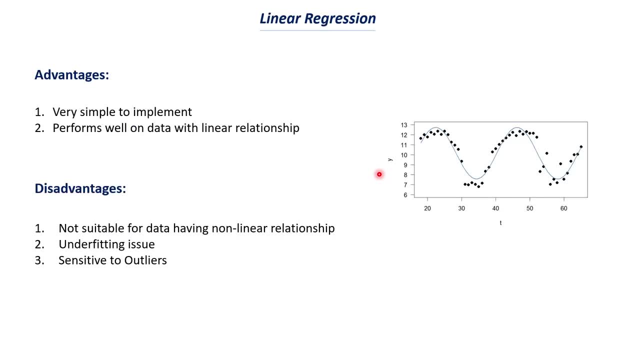 explain you how we can do this and you can, uh, do the research on other models, so we cannot go through all the models that we have. i'll just show this for the three models that we have. okay, so we know that linear regression is a very simple model and it is used for. 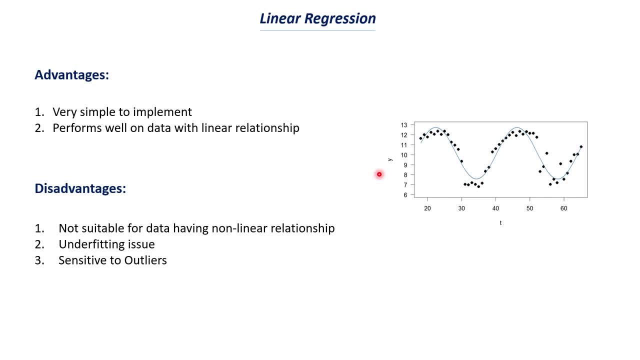 uh, linear regression tasks, okay, in other words, the regression problems. so the advantage of linear regression is like it is very simple to implement and the main advantage is it performs well-known linear relationship. linear relationship is in the sense like if, uh, the x value increases the y. 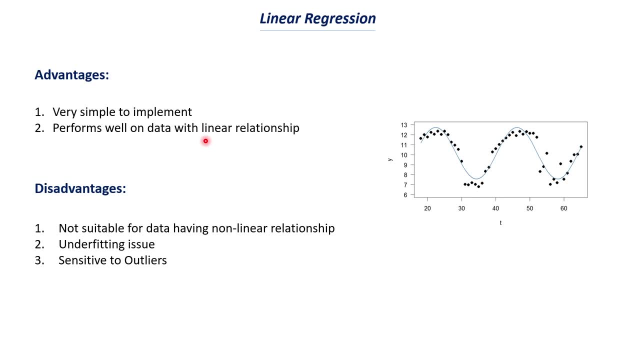 value also increases. if x value decreases, the y value also decreases. so that is only a linear relationship between them. so you can consider this: dsx and ys. you know it can be y. so if you see this curve, this is there is no, you know, a linear relationship between them. so it is kind of a. 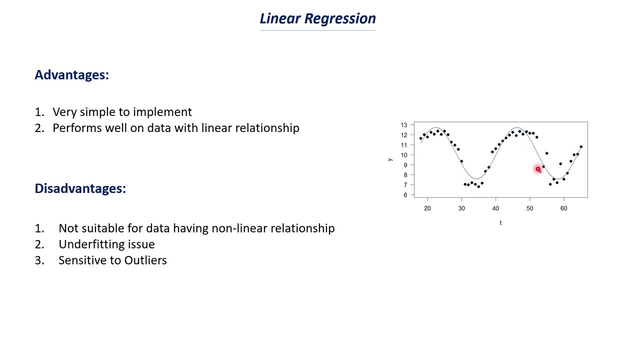 signed relationship, right. so like this is the curve you get for a sine function. so when the data is, uh, this kind of function, so you, in that case we cannot use linear regression, so it cannot capture that trend in the data, whereas if you have linear relationship in the data, in that case linear relationship, you know. 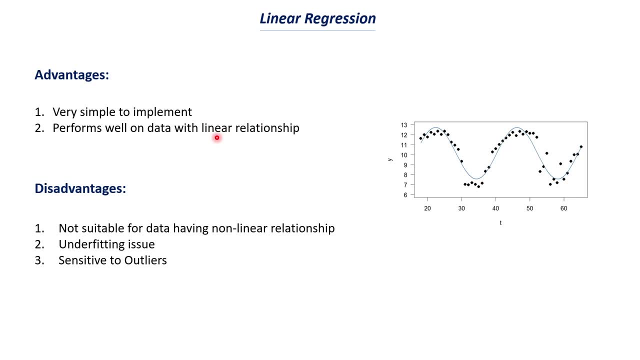 linear regression works well. so that is the main advantage of linear regression. so you can understand this, uh, the linear relationship using, uh, you know, the correlation matrix. so once you build this correlation matrix, you can put that in an eat map to understand whether there is some linear relationship within the data, within the different features, and so on again. so if you think, 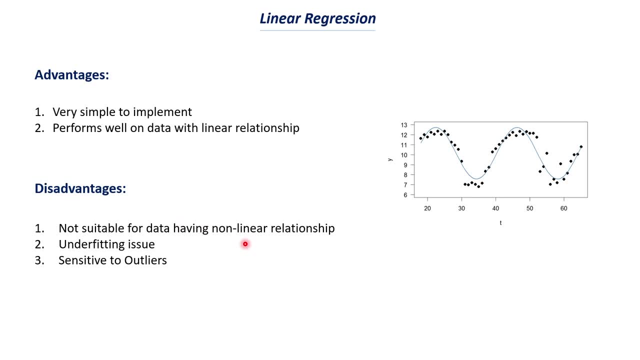 about the disadvantages. it is not suitable for the data having non-linear relationship. so when there is like uh, when there is no linear relationship in the data, when you use linear regression, you will get uh. you know the results won't be good, so there will be like uh, i error. 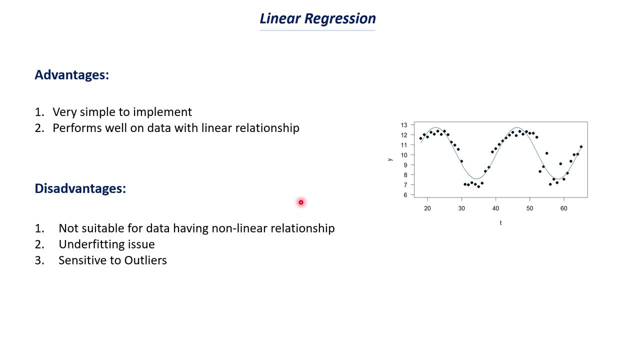 values. so we kind of try to avoid this linear aggressor. linear analysis is a very simple model okay, so we don't use it that much, but you know it's better to understand about this again. so it has this underfitting issue and sensitive to outlay. so this is another important factors. 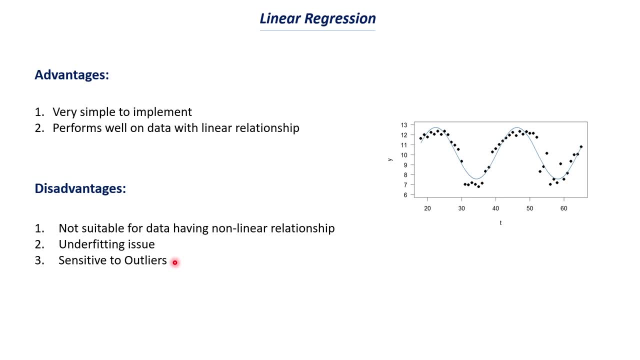 if you are at data as several outliers, then, uh, it is like it is best to not use a linear regression because, like linear regression, models are sensitive to outliers. so the function that we create using this linear regression is affected a lot by the outliers value. so we have to consider these things. 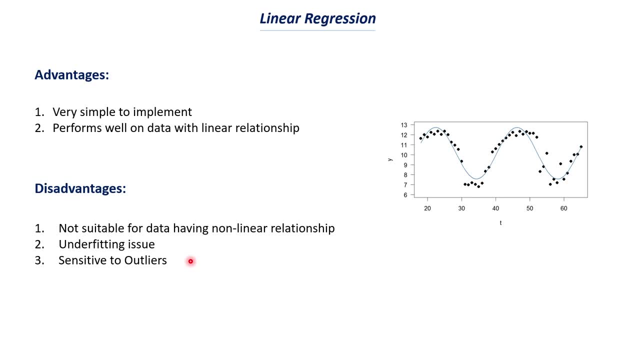 so like. so, if you think about different models, so this is how you can- uh, you know, evaluate on which model to choose. so you have to take into consideration both the advantages and disadvantages of a particular model and what is the data that you have. so, if you have, 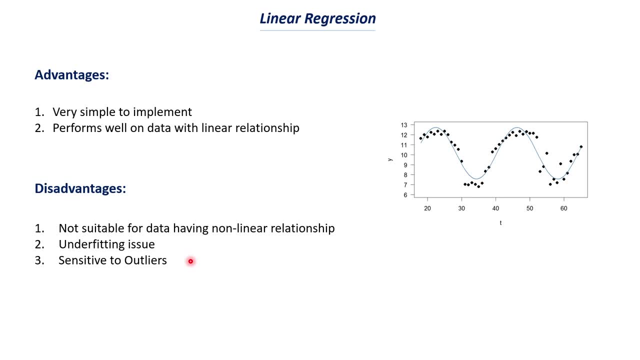 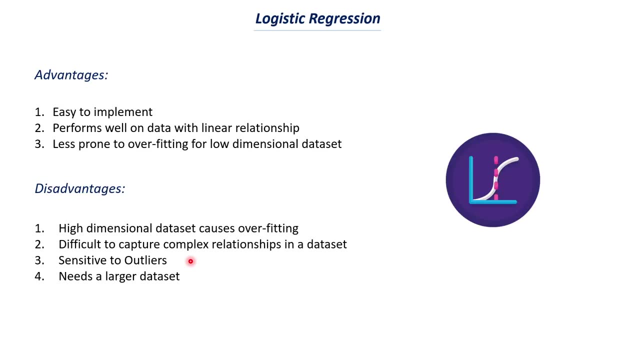 a linear data. it is not like that much complex and you don't have any outlays. you can go with linear regression. so you have to consider all these factors and you have to come to a decision. and if we talk about logistic regression, so we use it widely and again, so it is a very easy to 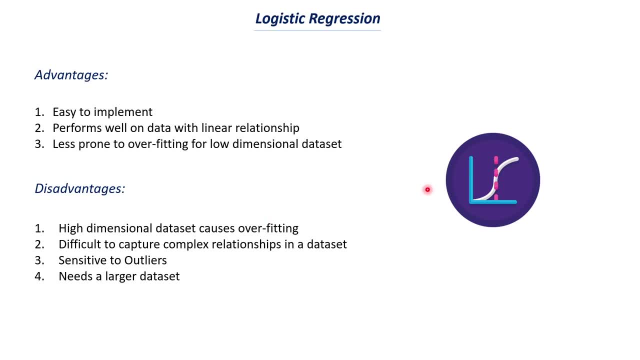 implement model. it is like a very basic model in machine learning and it is actually like built from linear regression. okay, so we take the linear regression function and we apply the sigmoid equation. okay, so that's why, that's how we get this logistic regression model and, yes, this logistic. 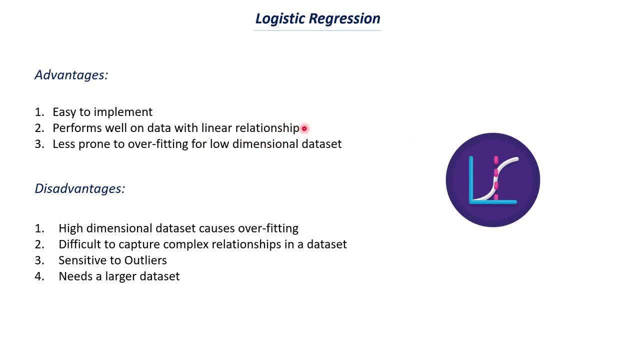 regression also performs well only on the linear relationship data and again, it is used only for binary classification problem. it can't be used- you know that, efficiently for multi-class classification or regression problems. you cannot use it, but for binary classification problem where the data has a linear relationship between them. in that case we can use logistic regression. it is a very good 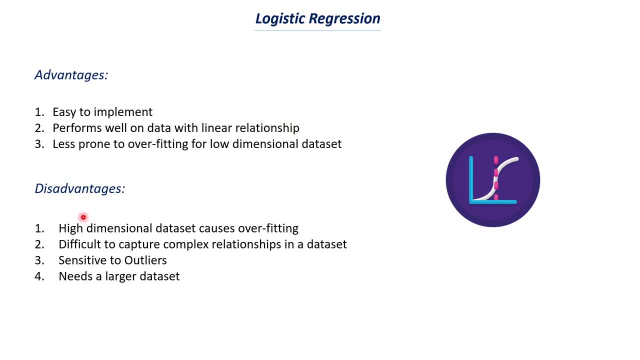 model and so if we consider about disadvantages, like if the dimension uh within the data is very high, in that case logistic regression won't perform well. so there will be this overfitting dimension in the sense when you have uh, when the number of columns is very high in our data set. so 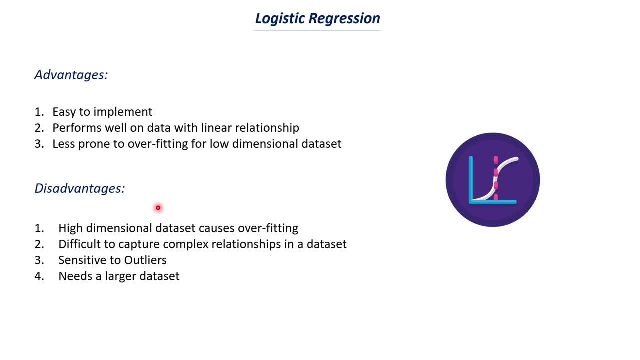 in that case, logistic regression won't work well. so you have to look at the data and and see whether, okay, whether we can, you know, use the logistic regression in this case, or i have to go with support detector machine or random forest classifier and so on. so if the dimension is more, 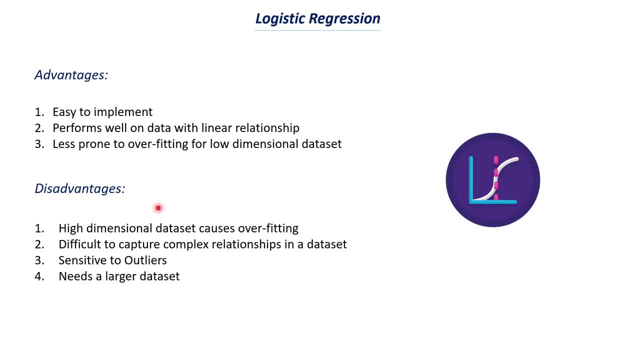 more often support classifier used because, like it kind of uh works well on high dimensional data. so that is one thing and uh again. so if, like this logistic regression, it is difficult to capture complex relationship, again it is based on linear uh regression, so it works well only on the. 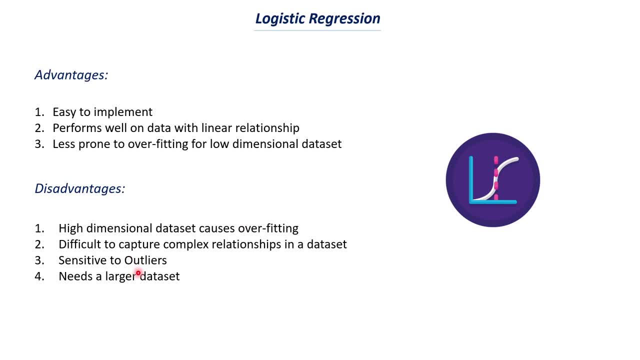 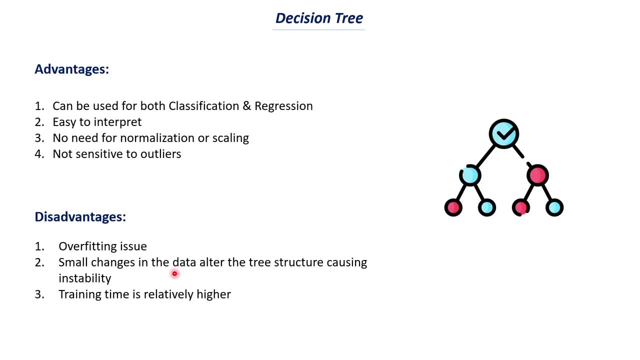 uh, data set which has linear relationship between them. again, this is sensitive to outlay outliers and it needs a larger data set, so small data sets it cannot capture that trend properly, and so on, and this is the last model that i will discuss. so remaining models. you can do your research on what. 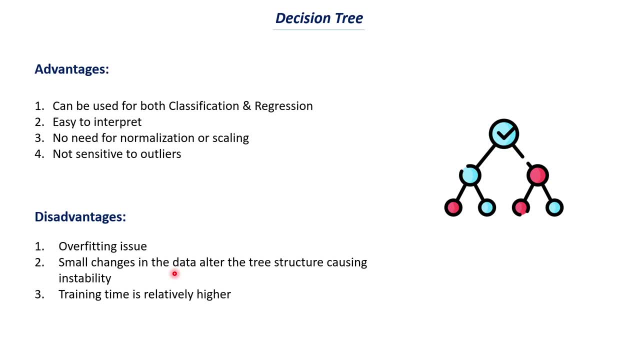 is what are all the different advantages that you have and the disadvantages that you have, and so on. i just wanted to give you an idea of how you can look at this advantage and how you can select the model. okay, so, if we talk about logistic regression, we can look at this advantage and how you can select the model. okay, so if we 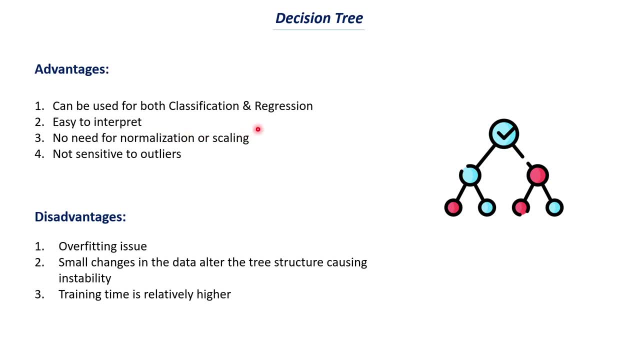 talk about decision tree. it can be used for, again, both classification as well as regression, and it is like easy to interpret. so we have this decision on notes, or what we call as uh. you know, so we have the branches and we have like two nodes and each note, like uh, will add two. 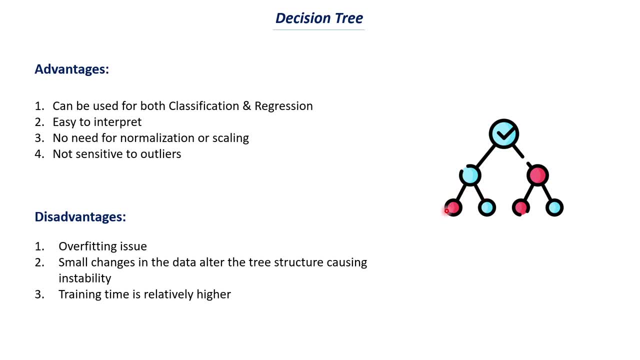 outcomes. so it can be like yes or no and if the answer is yes, it will go to one branch and the answer is no, it will go to the other branch. so we have seen this in decision tree intuition video and so on. i hope that you have seen that video so like. it is like easy to interpret and understand. 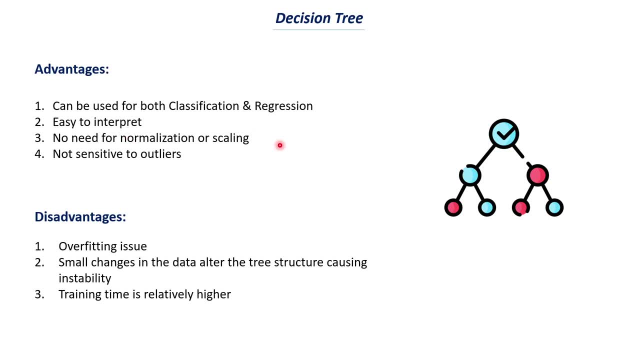 and like no need for normalization or scaling. so normalization is uh, when we try to convert all the columns so that all the values are in the same range. so that is what we call as normalization and we, so we have this scaling rate. so what the standard scale does is, it will try to uh bring. 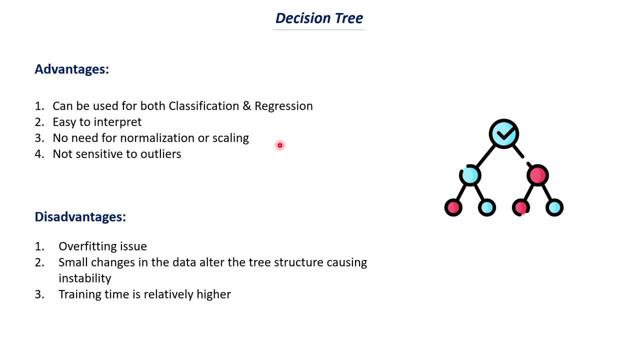 the data to a normal, normal distribution, you know. so that's what the standard scale does. so when we are working with the regression model, we have to do this normalization and scaling, whereas for the and random forest models. so, if we want, we can skip these steps because the this tree based. 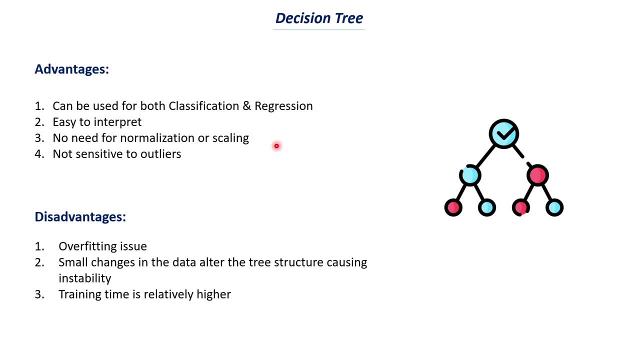 models can understand the data without normalizing or scaling and again, so these are like not sensitive to outliers compared to the regression model. so, if you like, this is like a very, very important thing, like this particular question can also be asked in interviews as well, so they: 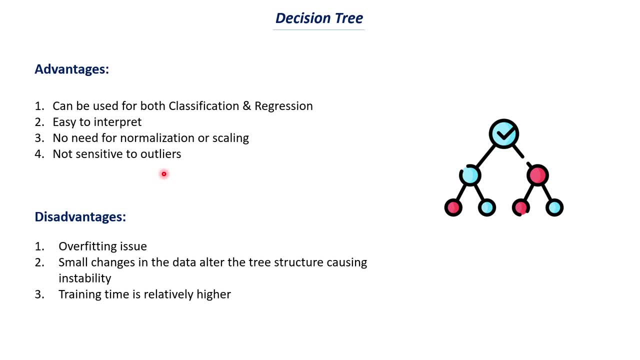 would ask like: which model is not sensitive to outliers? so the correct answer would probably be tree based models, whereas regressors are greatly affected by the outliers. so the linear regression, lasso regression and so on, so these decision trees are not affected by outliers. so if you 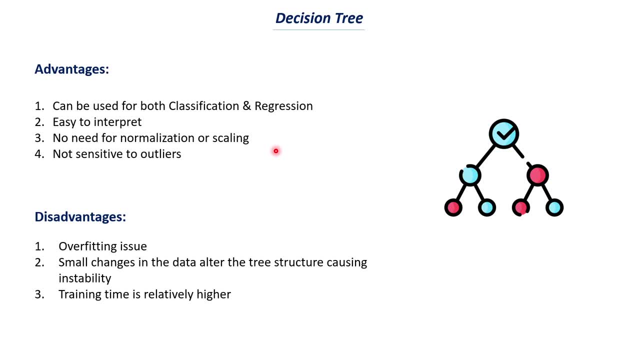 have a data set and there are like several, like a few outliers are there. so if you don't want to process the outliers, you can directly use the models, like decision trees or random forest. but if you want to use a regression model, you have to process this outliers before using them. so this is 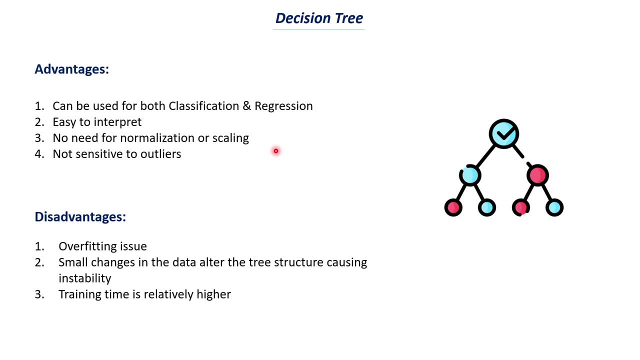 like the other thing that you can consider while selecting the model. so if we consider about the disadvantages of this decision tree model, then we can say that the outliers are not sensitive to the decision tree, so it has this overfitting issue where you will get high accuracy for training data. 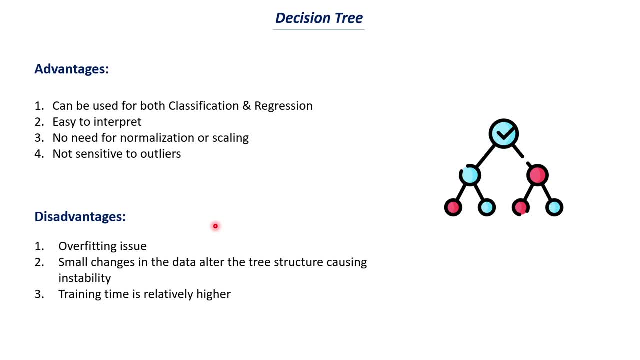 but the accuracy and test data will be low and, again, small changes in the data may alter the tree structure, causing instability. instability means, like you, may get different results because, like you know, if if the values are like changed by a small factor, then the result will change by a 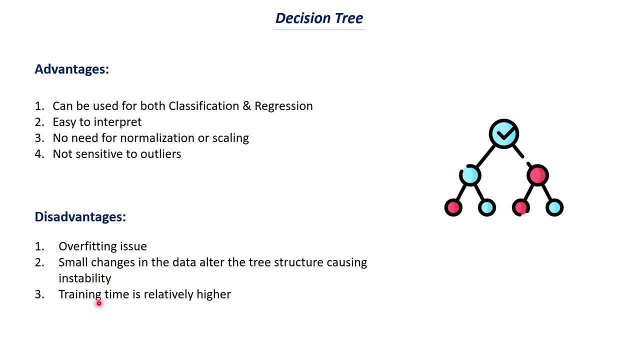 huge factor. so that's what i mentioned by this second you know disadvantage. and the third main disadvantage is the training time is relatively higher. so the amount of time the model takes to train and when you take a new data set, you can get a lot of results and you can get a lot of results. 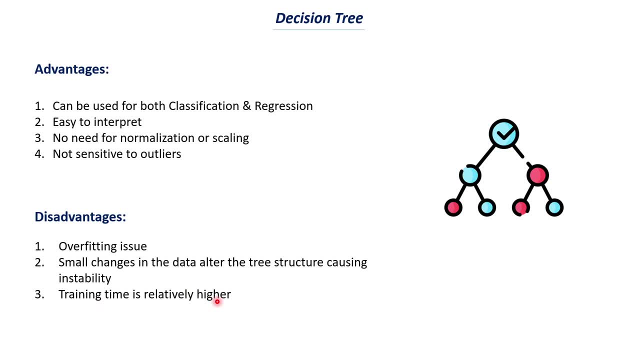 and if you want to predict the label for the new data point, it is going to take a somewhat longer time compared to the other models. so this is something that is like very crucial, because if you have a data set that has 500 data points or 1000 data points, that's not an issue, but if you 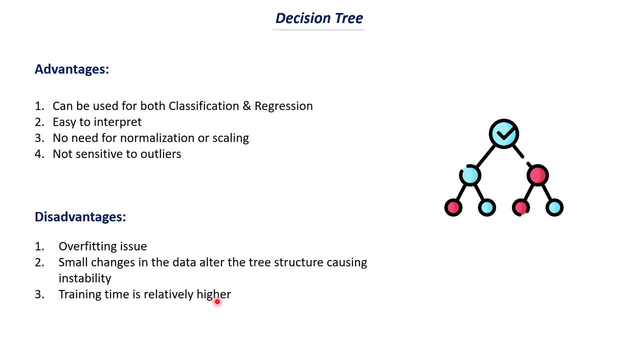 have a data set that has, like, let's say, a million rows. in that case, if you're going with the pre-based models, it will. it will probably take a very long time. so these are like different factors that we have to consider, and this will help us to choose the best model for our particular use case. so i